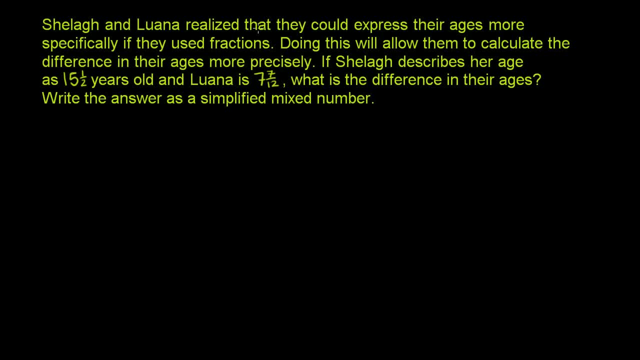 Sheila and Luana realize that they could express their ages more specifically if they used fractions. Doing this will allow them to calculate the difference in their ages more precisely. If Sheila describes her age as 15 and a half years old and Luana is 7 and 7 twelfths, I'm assuming- years old, what is? 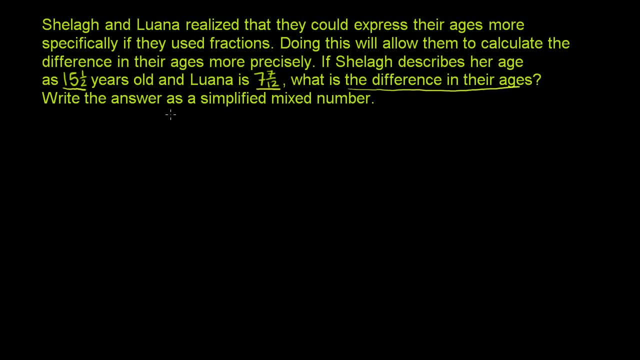 the difference in their ages. The difference in their ages. Write the answer as a simplified mixed number. So Sheila is older, So she's 15 and a half years old. So we really want to find the difference between 15 and a half and 7 and 7 twelfths. 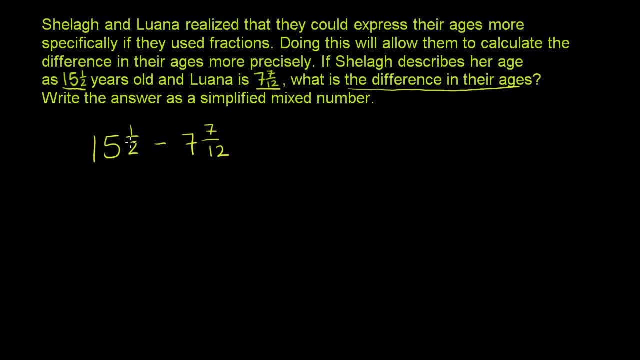 And we could see immediately. or maybe it's not obvious to you, but 1 half is the same thing as 6 twelfths, which is less than 7 twelfths. So if we separate out the whole number parts and the 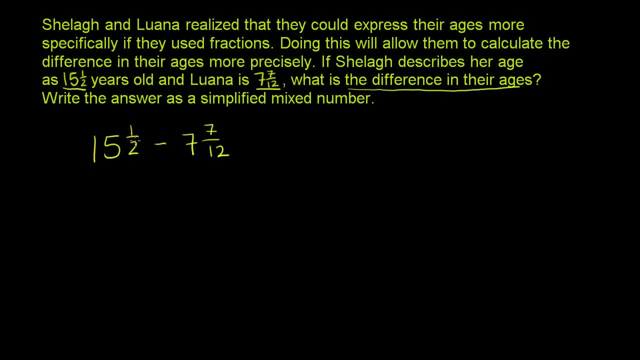 fraction parts. this fraction is actually smaller. The 1 half is smaller than the 7 twelfths, So it might be easier to just do this. Let's write both of them as mixed numbers, so we don't have to do all of that borrowing and regrouping. 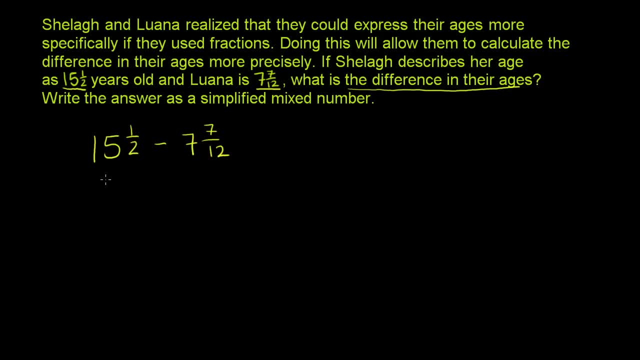 So let's write both of them as mixed numbers. So we have 15 and 1 half. Let's write both of them as improper fractions. So we're going to keep 2 in the denominator And as an improper fraction, 2 times 15 is 30, plus 1 is 31.. 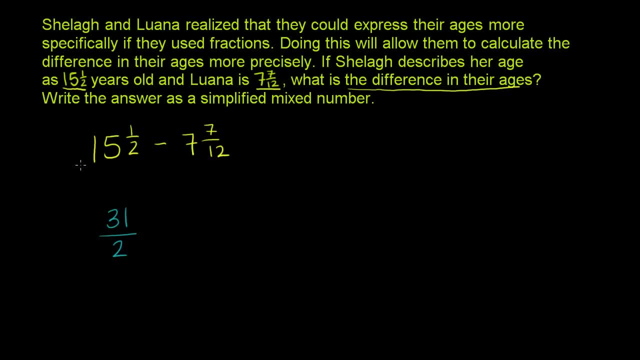 So 31 over 2 is the same thing as 15 and a half. So these are equivalent. And then 7 and 7 twelfths, If we write it as an improper fraction. So we're going to still have the minus sign out there. 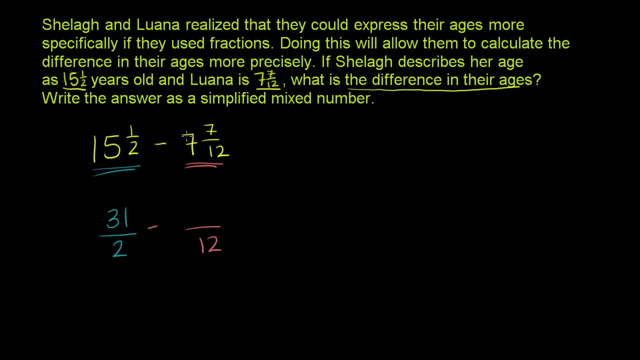 The denominator is 12.. 12 times 7 is 84.. 84 plus 7 is 91. It is 91.. Did I do that right? 91.. Yep, that looks right: 91 over 12.. Now we've written both of them as improper fractions. 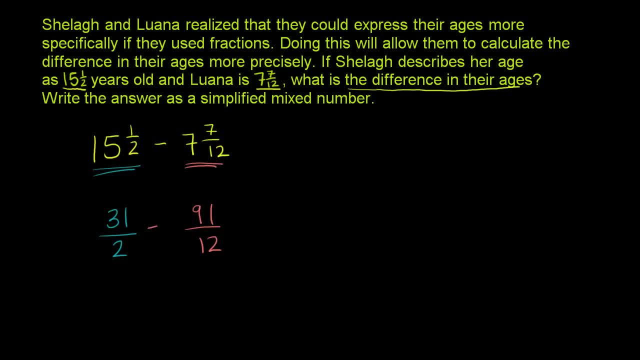 but we still have different denominators, So we have to have a common denominator. So what is the least common multiple of 2 and 12? Or what's the smallest number that's divisible by both of them? Well, 12 is divisible by 12, and 12 is also divisible by 2.. 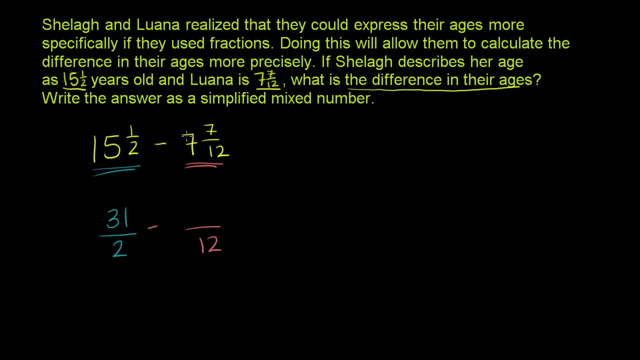 The denominator is 12.. 12 times 7 is 84.. 84 plus 7 is 91. It is 91.. Did I do that right? 91.. Yep, that looks right: 91 over 12.. Now we've written both of them as improper fractions. 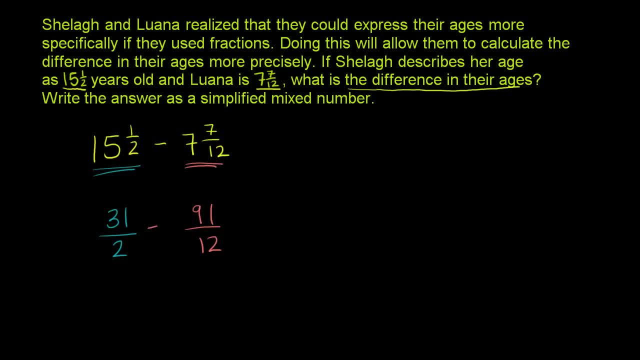 but we still have different denominators, So we have to have a common denominator. So what is the least common multiple of 2 and 12? Or what's the smallest number that's divisible by both of them? Well, 12 is divisible by 12, and 12 is also divisible by 2.. 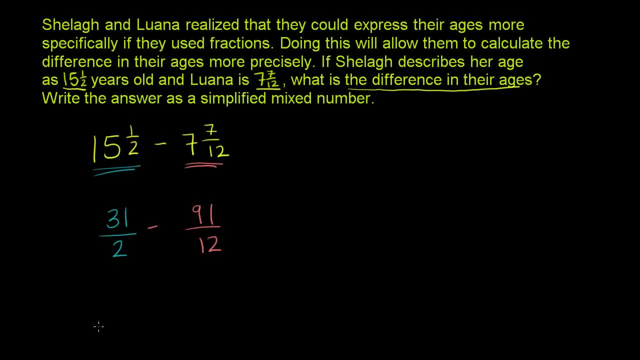 So 12 is the least common multiple. So we want both of them to be over 12.. And this fraction already is over 12, so we don't have to change it: 91 over 12.. Now on the blue one, to go from 2 to 12 in the denominator. 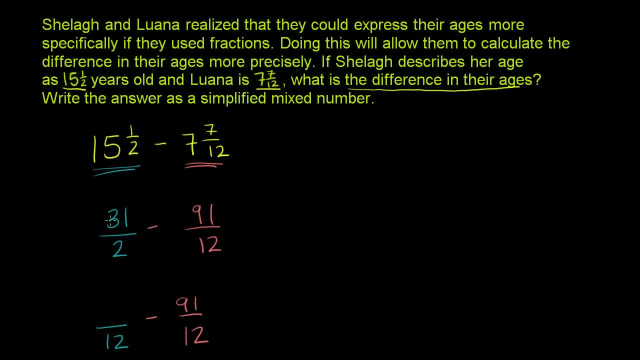 we have to multiply by that, It's going to be 6.. So we also have to multiply by 6 in the numerator. So if we multiply 31 by 6, what do we get? And you can even do this in your head. 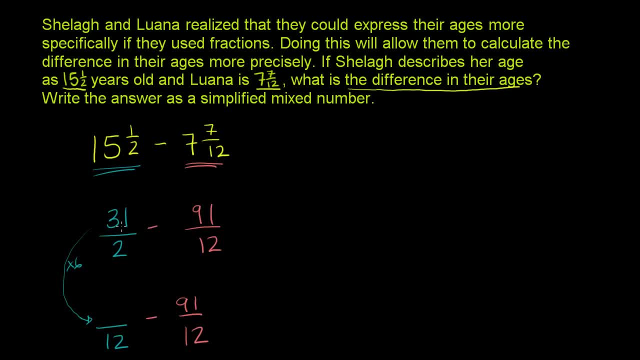 6 times 30 is 180.. 6 times 1 is 6.. So it's going to be 186.. And now we subtract. So the difference in their ages is going to be The denominator is going to be 12.. 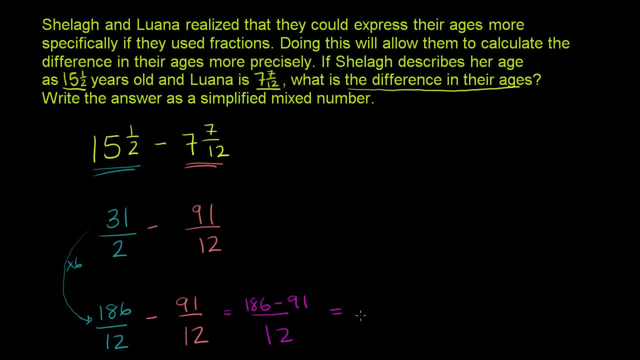 It's going to be 186.. 186 minus 91,, which is equal to over 12.. See: 186 minus just 90 would be 96.. We're subtracting 91,, so it's going to be 95.. 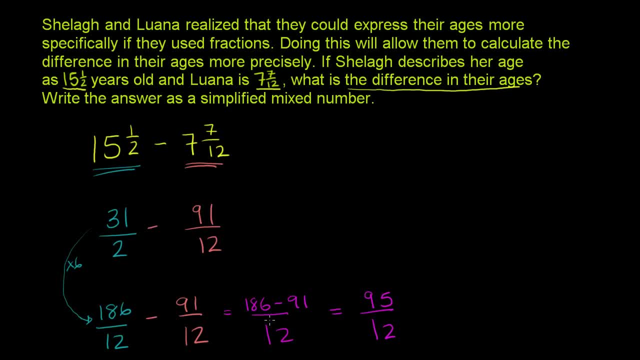 6 minus 1 is 5, and then 180 minus 90 is 90.. So that works out. So the way we've expressed it right now. it is an improper fraction, but they want us to write it OK. 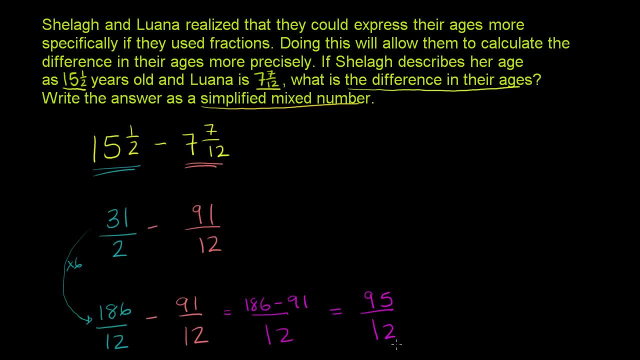 They want us to write it as a simplified mixed number, So let's do that. So how many times does 12 go into 95?? Let's see, 8 times 12 is 96. So that's too big. So 12 goes 7 times. 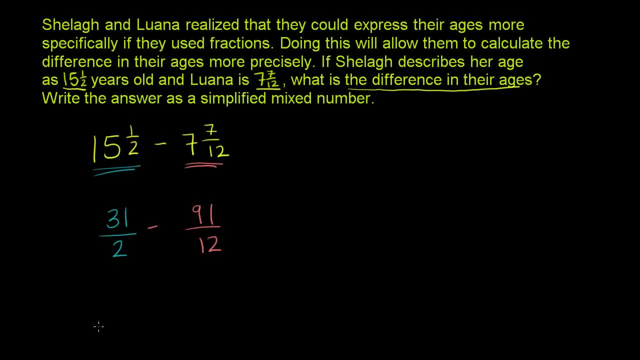 So 12 is the least common multiple. So we want both of them to be over 12.. And this fraction already is over 12, so we don't have to change it: 91 over 12.. Now on the blue one, to go from 2 to 12 in the denominator. 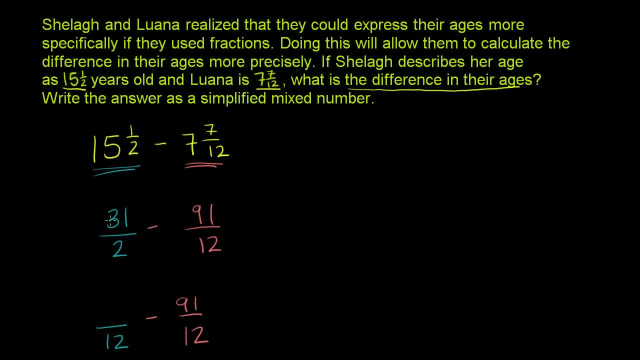 we have to multiply by that, It's going to be 6.. So we also have to multiply by 6 in the numerator. So if we multiply 31 by 6, what do we get? And you can even do this in your head. 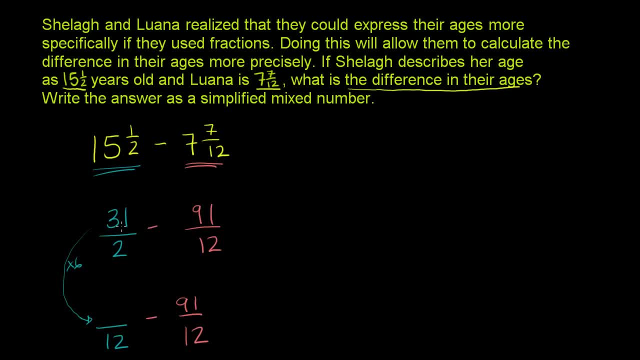 6 times 30 is 180.. 6 times 1 is 6.. So it's going to be 186.. And now we subtract. So the difference in their ages is going to be The denominator is going to be 12.. 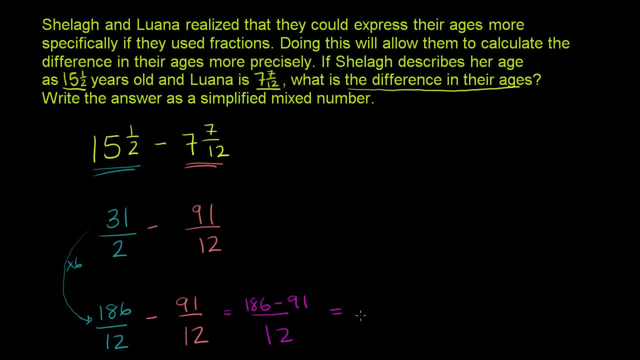 It's going to be 186.. 186 minus 91,, which is equal to over 12.. See: 186 minus just 90 would be 96.. We're subtracting 91,, so it's going to be 95.. 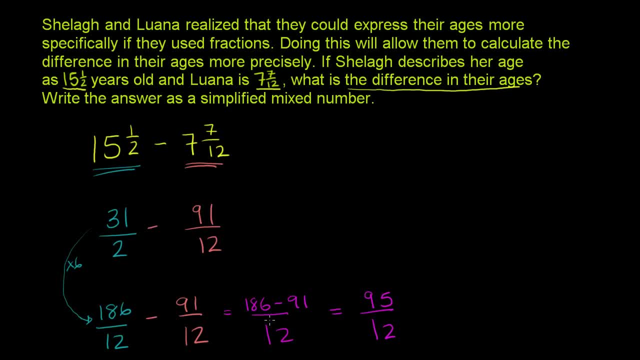 6 minus 1 is 5, and then 180 minus 90 is 90.. So that works out. So the way we've expressed it right now. it is an improper fraction, but they want us to write it OK. 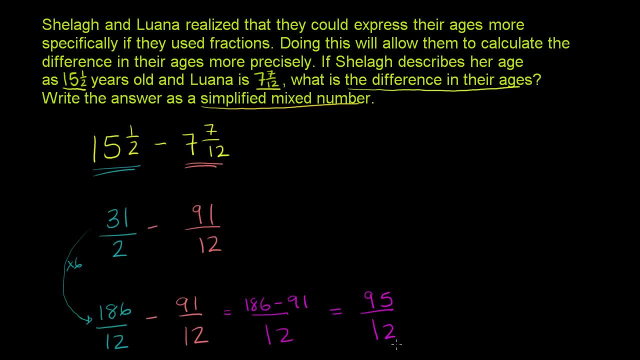 They want us to write it as a simplified mixed number, So let's do that. So how many times does 12 go into 95?? Let's see, 8 times 12 is 96. So that's too big. So 12 goes 7 times. 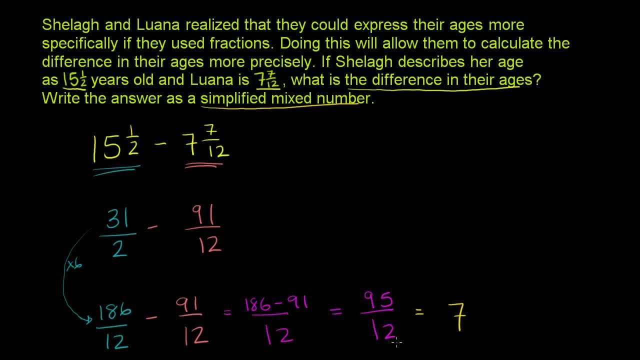 So this is equal to 7.. Let me write it out, We don't want to do too much in our head. If we go 12 into 95, I'm saying it goes 7 times. So if that's true, If that's the largest number, then the remainder. 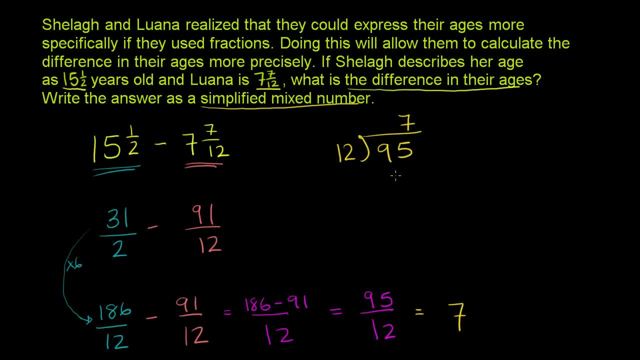 should be less than 12.. 7 times 12, we know, is 84 from our times tables. Or you could just think it's going to be 14 plus 10 times 7, which is 70. Either way, And let's see 95 minus 84.. 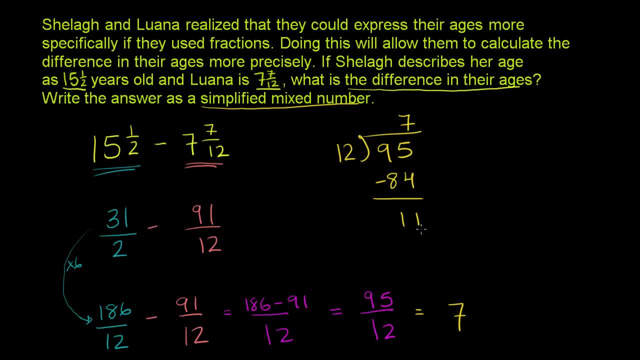 5 minus 4 is 1.. 9 minus 8 is 1.. So we have a remainder of 11.. So 12 goes into 95. 7 times You get 7 wholes and you have 11 left over.